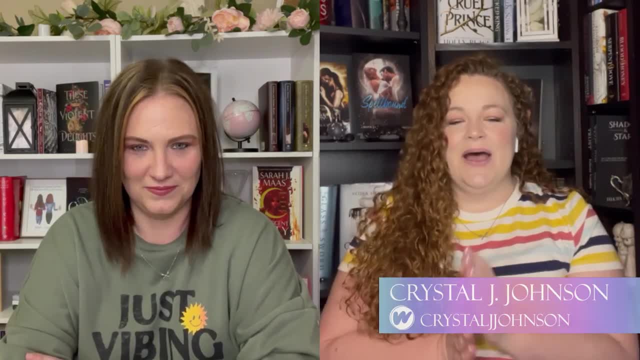 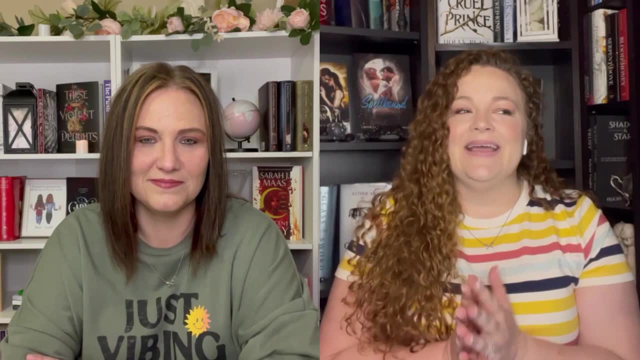 Crystal. That is The Shadows Between Us. Yes, by Trisha Levenseller. That is what got us on this kick to talk about morally gray characters. So if you want to read any of those stories, we'll see. ya, We'll see you next time. 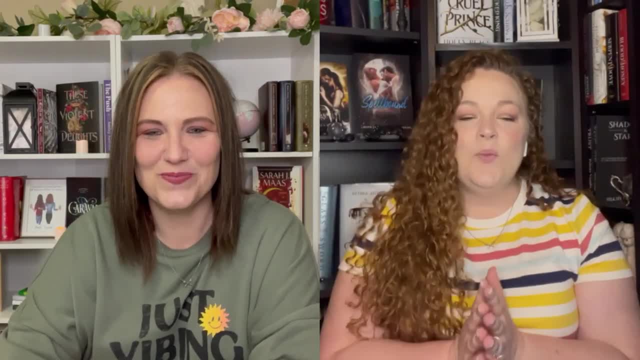 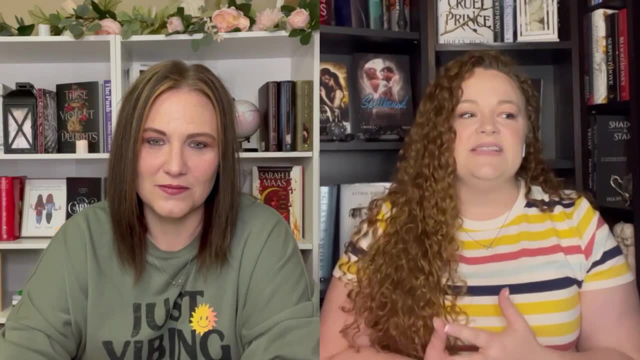 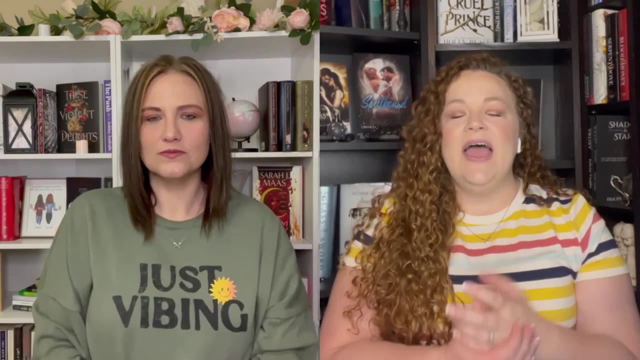 All right, so let's get into it. Why did a book that is so popular on TikTok, The Shadows Between Us, start all this? And that's because I read this story and it's the main characters, It's Alessandra and the Shadow King. They are presented as morally gray characters. 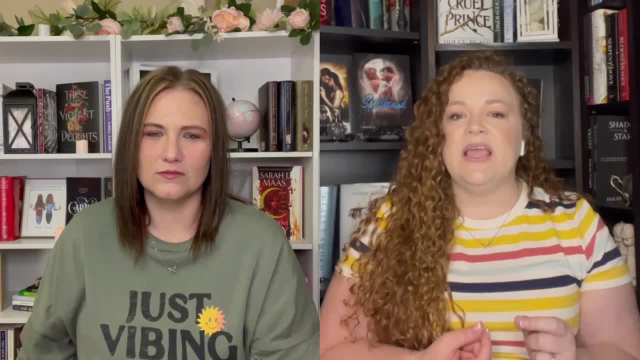 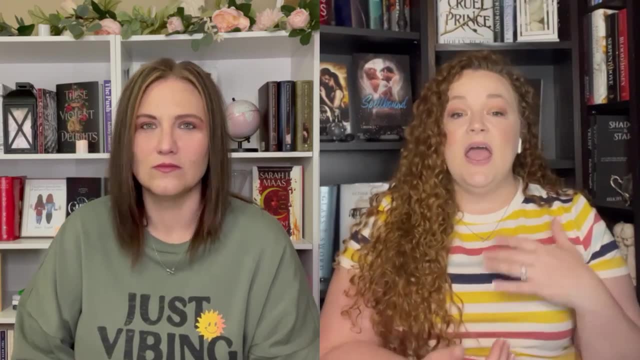 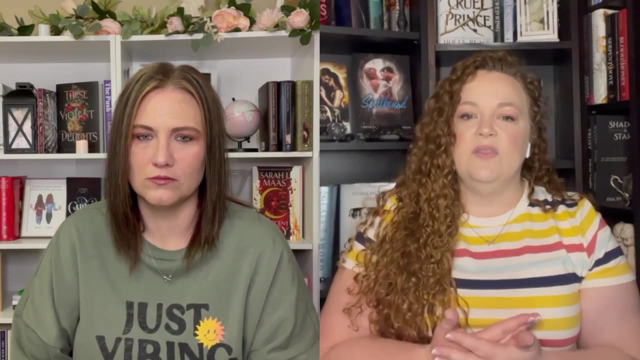 but there is something missing here and that is their likability, And for me, if you love this book, by all means, that's your opinion, This is my opinion and why I really had trouble connecting with the story, And that is because they, in so many ways, were not living in the gray. 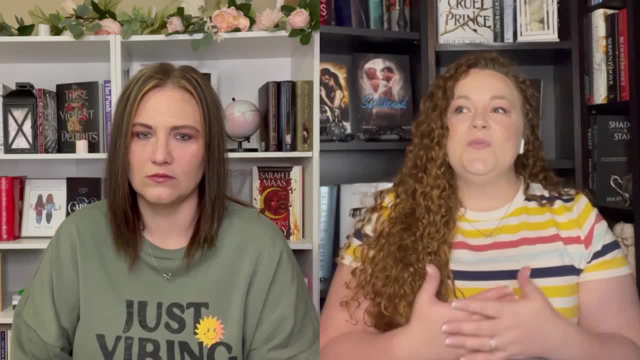 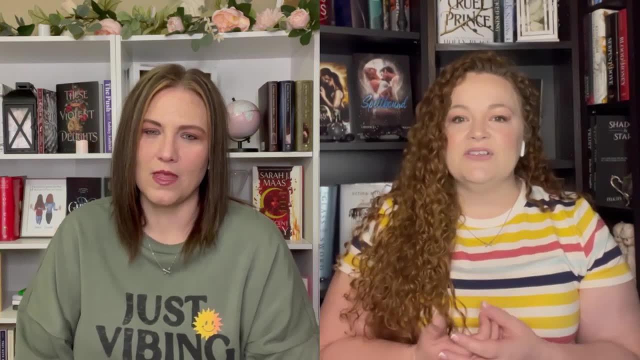 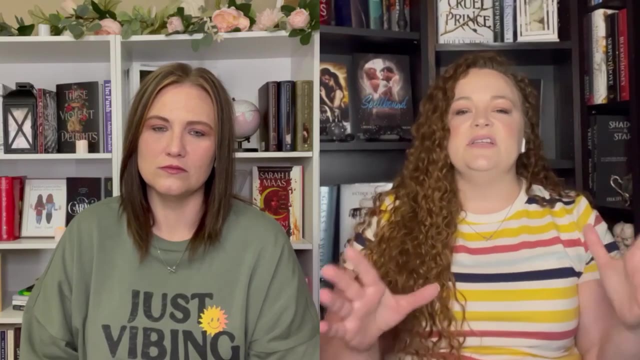 And part of living in the gray is justification. There was none, And therefore they just become these dislikable characters for me. So if you've not read it and or don't have any clue about it, the oldest sister kind of gets all the attention until the time comes that she's been promised to marry. 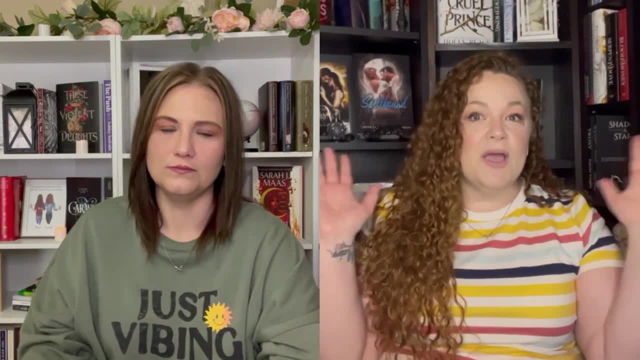 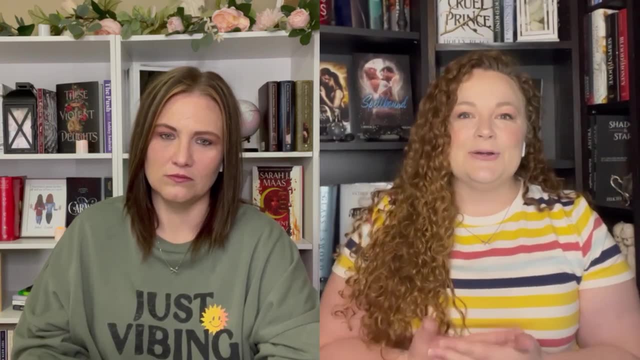 And now it is Alessandra's turn and she's going to go for the big one. She's going to take the shadow king and Kill'em and take over his kingdom, and that is her driving force. And the shadow king isn't the shadow king, is he? 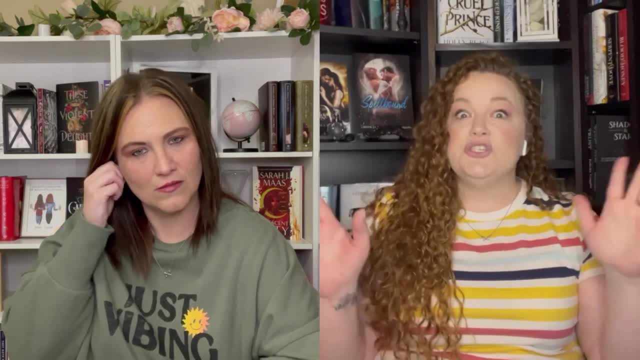 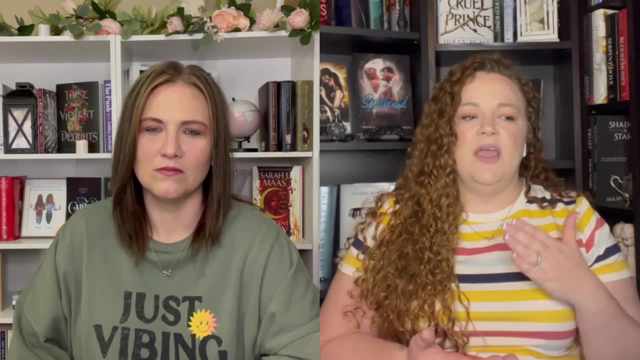 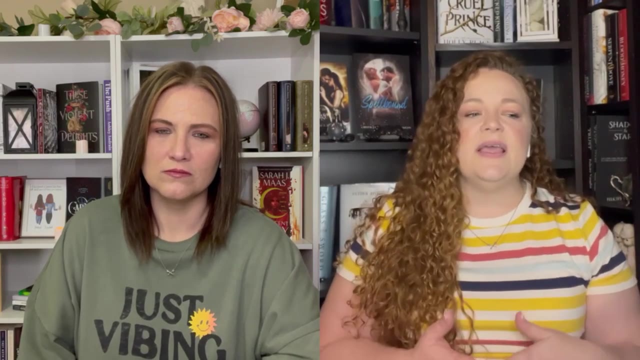 king. he doesn't allow anybody to touch him, he's got shadows, and there is one particular scene that I just could not get over it. whenever I think of this story, it sticks with me and it's this moment. there is this person that is out to kill the king and he gets by and gets close to Alessandra. 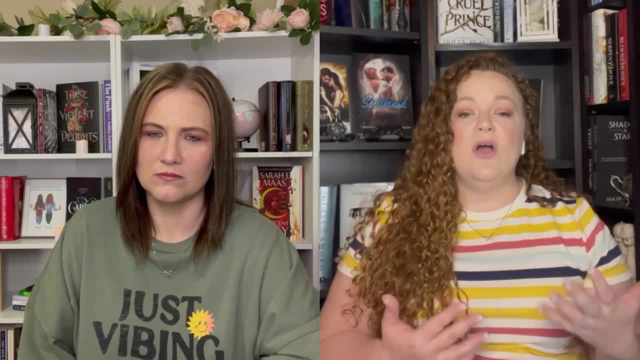 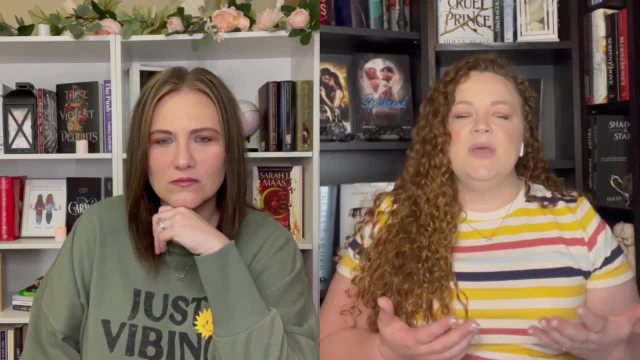 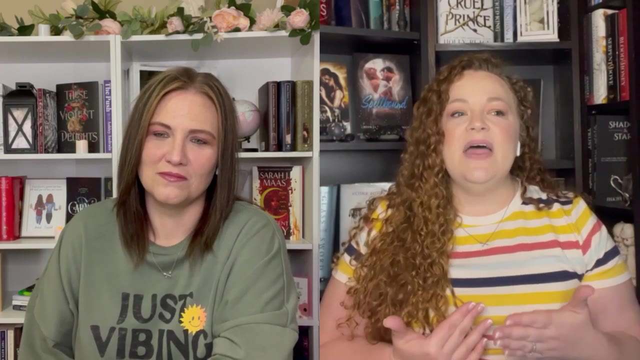 and the king at one point when they're out on this picnic and the guards are weren't paying attention and the king's really pissed and one of the guards is out picking flowers for the woman he loves. granted, he wasn't doing his job, but I mean the king kills him and then she's like well. 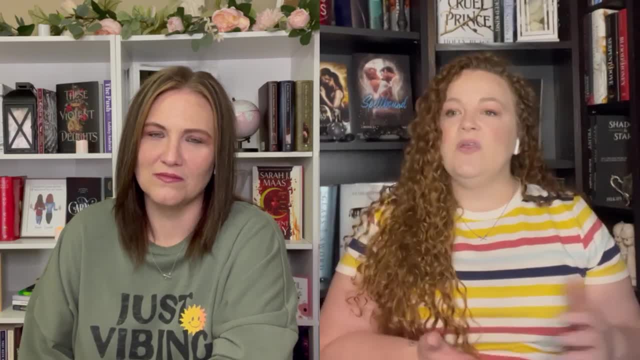 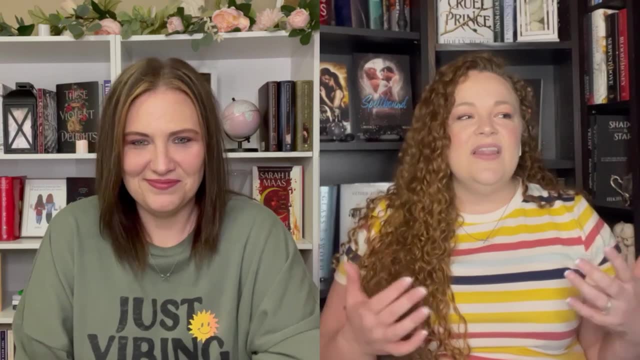 Alessandra asked: are you going to kill the other ones because you only killed one of the guards? he goes: well, we need somebody to get us home. as soon as we get home, I'm killing them all and I just felt like I get you gotta make a. you're a king, people need to. 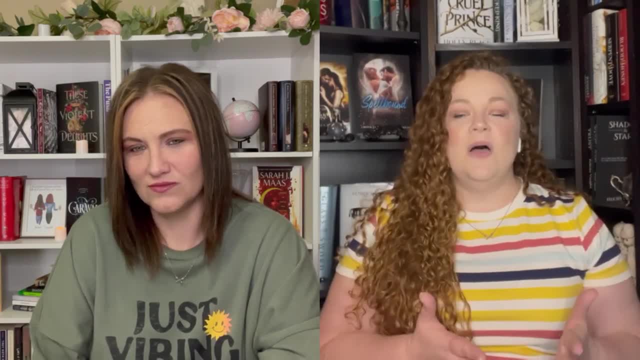 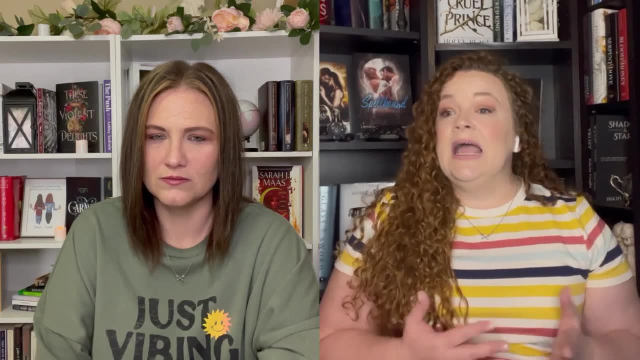 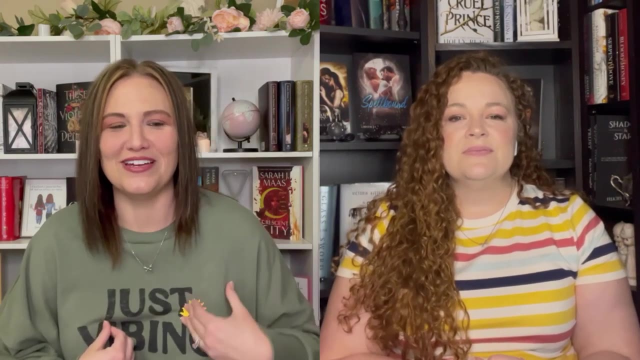 be where they need to be and taking care of you and watching over you. that is their jobs. but, holy smokes, you're gonna kill them. there's just nothing likable. he's not like a likable ruler. I hated him. we want. we're taking this as an excuse to talk about some of our favorite. 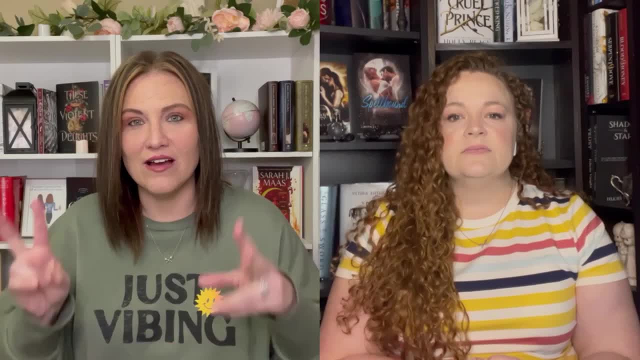 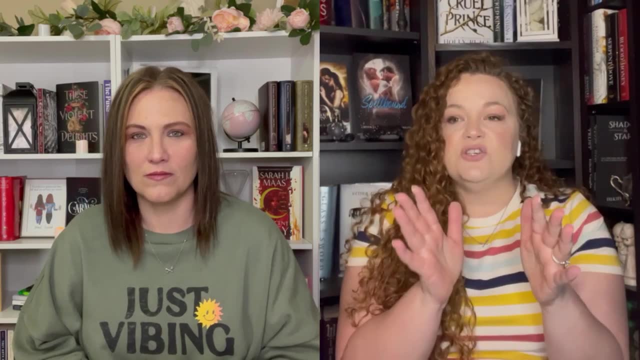 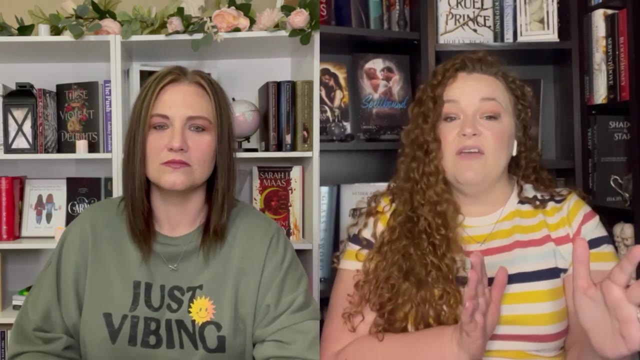 characters, but also tell why their morally grayness is okay works, why they're bad, like the things they do that on a moral spectrum are terrible, why they're not doing their job is the why of them. yeah, this is why we forgive them. there's nothing that I forgave about Alessandra. 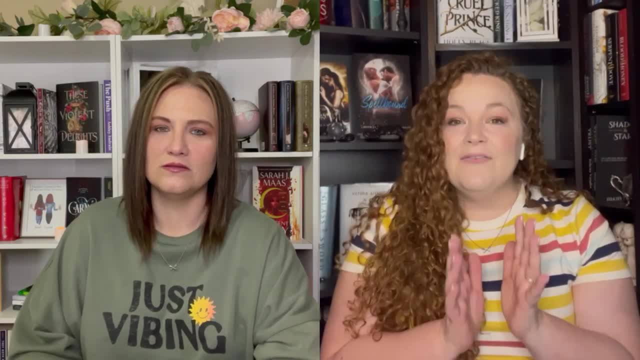 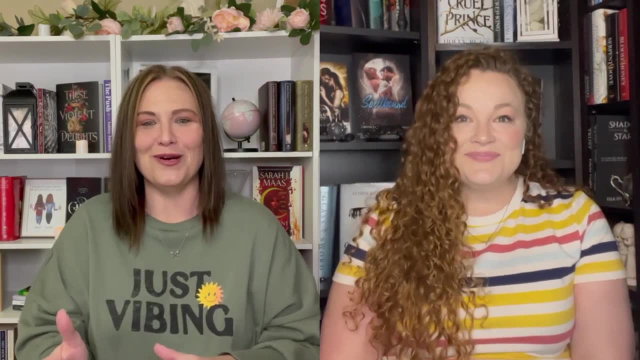 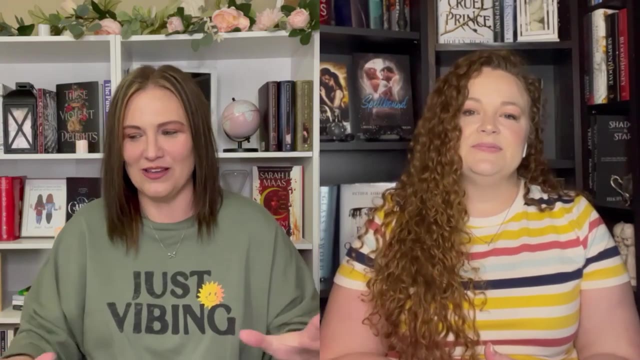 or the shadow king. these characters have reasonings behind them that are forgivable, so here we go. okay, the first one we're gonna talk about is one of our very favorite book boyfriends ever, and that's Rhysand. we talk about him all day, but what we're here to talk about is the questionable he. 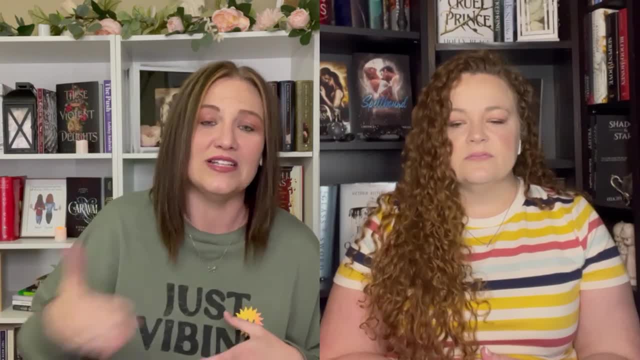 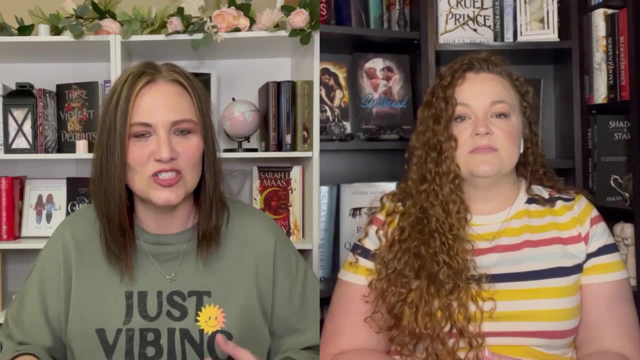 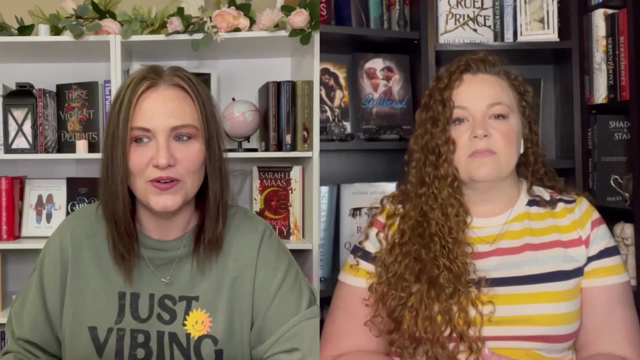 does at the end of A Court of Thorns and Roses and at the beginning of the second, which is A Court of mist and fury. he does do some questionable stuff but in the end, when everything is explained, he had the best reason for doing the things that he did. he did it to protect all of his people in 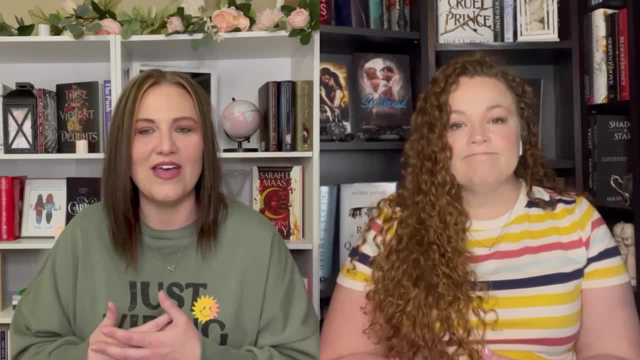 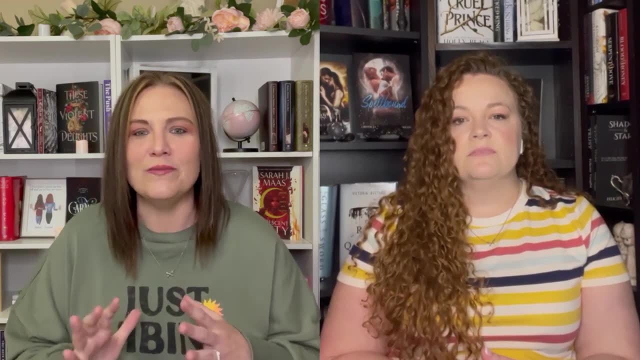 his in his court, like the people that he ruled. if he hadn't done that, they would have all been dead- and the things that he did to pharah- he was doing for her so that she wouldn't have to remember all of the terrible, terrible stuff that was happening. because he loved her, he already knew that they 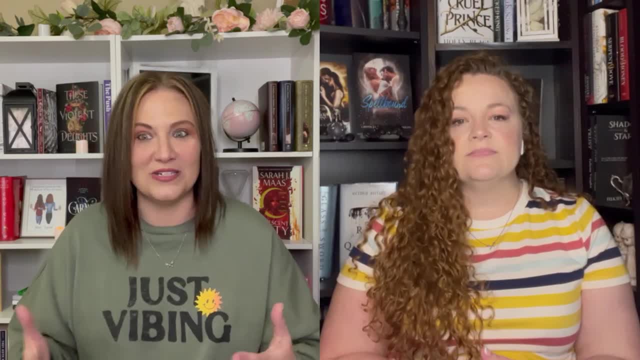 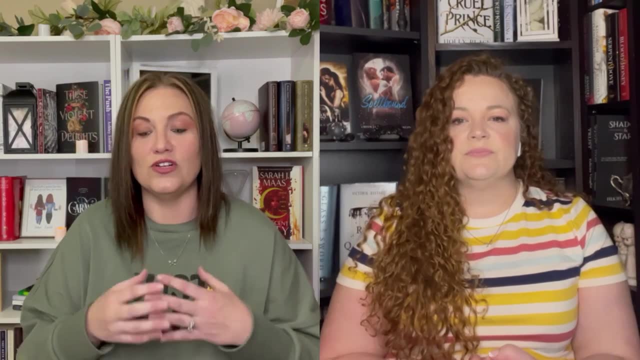 were mates, so he was doing everything he could to to protect her. and once all of that is explained, you're like: oh okay, that makes sense. everything he did was for the greater good of the innocent people, so we can forgive some of the questionable things he did. actually, i 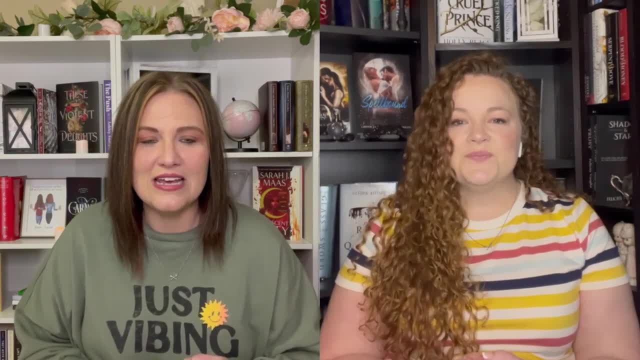 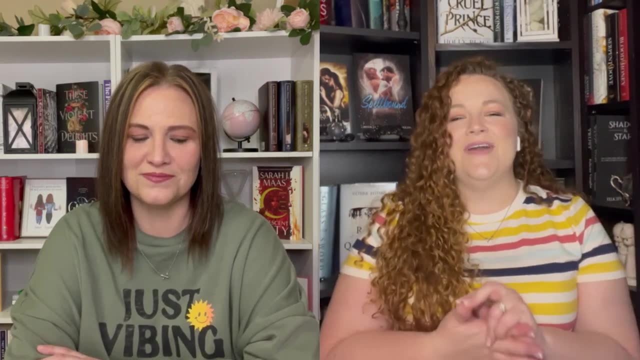 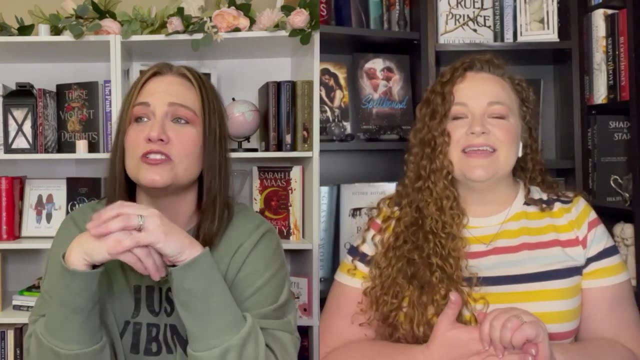 forgave all the questionable things he did, and most of the questionable things he did he didn't even do. they were easily explained. number two is hawk from from from blood and ash by and unreal arm and trout. big spoilers ahead, a huge. just go ahead and stay here, castiel the dark. 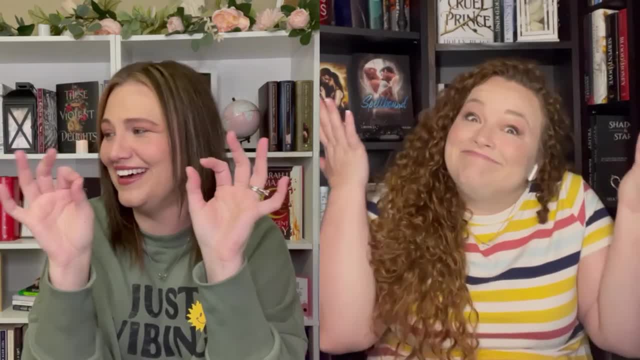 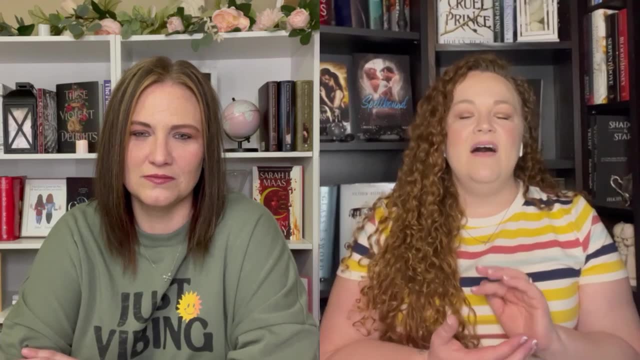 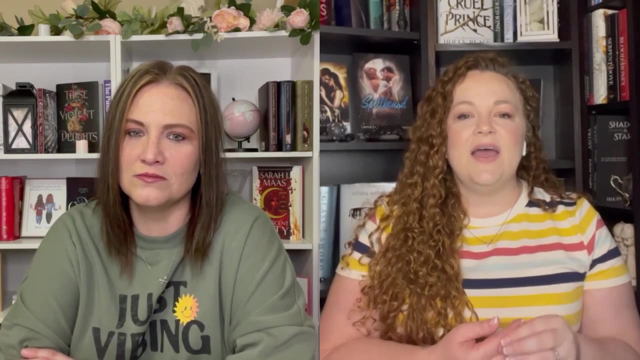 one. okay, castiel, the dark one, if you're still watching, it is your fault. we tried to tell you the great thing about this story is the idea of perception, and when people are feeding you your perceptions of things, how you're not seeing the whole story, even when it's not feeling right and 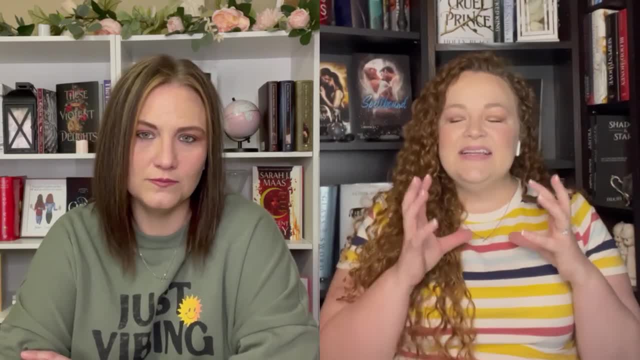 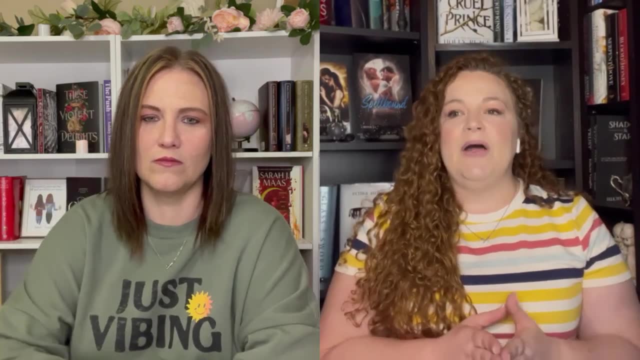 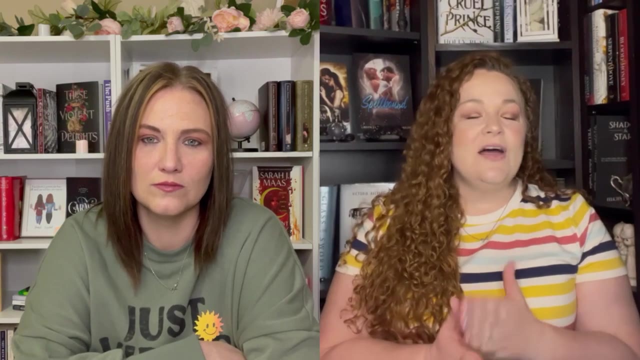 this in life all the time, and it is really well done in this story, because you start to learn that everything that poppy thought she knew about the craven, about the atlanteans, about everything- is not what she thought it was and she thought she was on the side of the good guys the entire time. 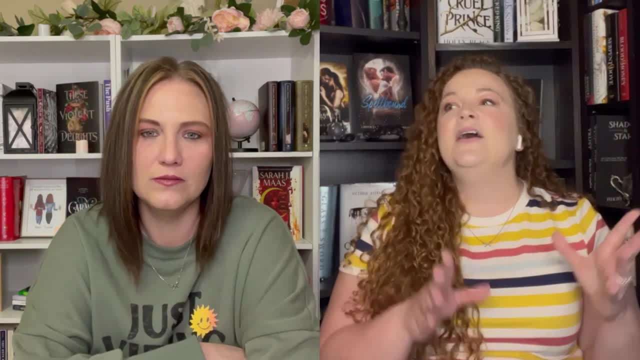 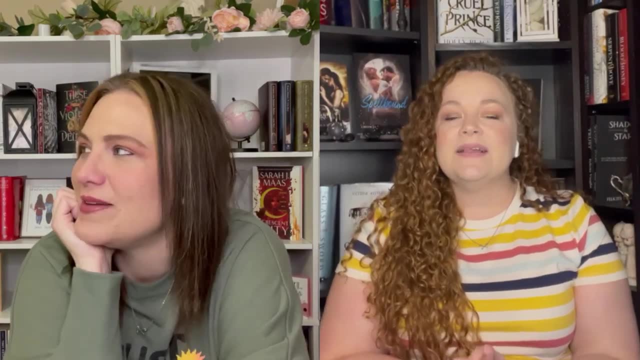 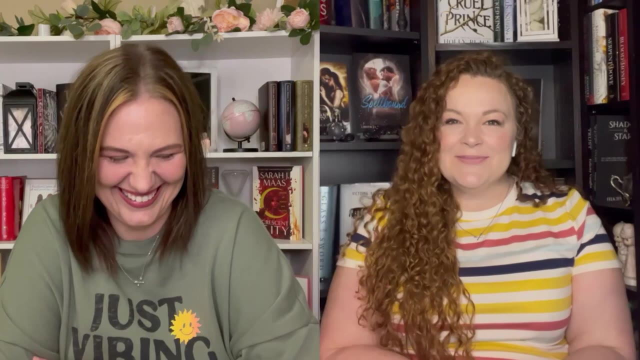 and it turns out, when you get all of castiel hawk- whatever you want to call him today, we call him both, because he likes both names. we could also. we could also call him daddy, if that's your thing. no judgment, just kidding, just kidding. we realized that everything he was doing, even his intentions- 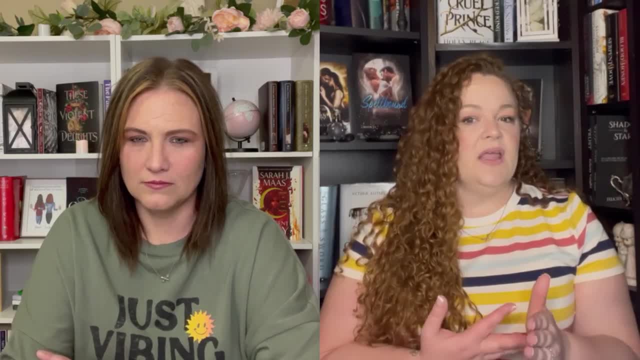 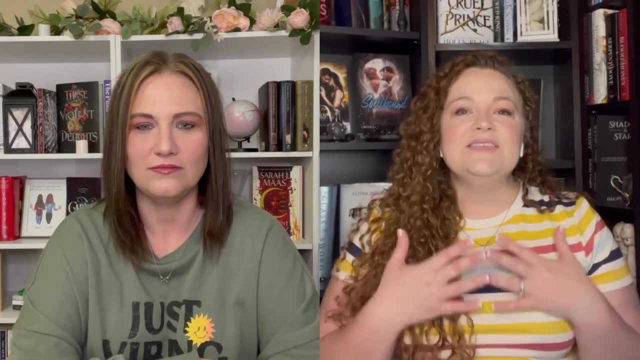 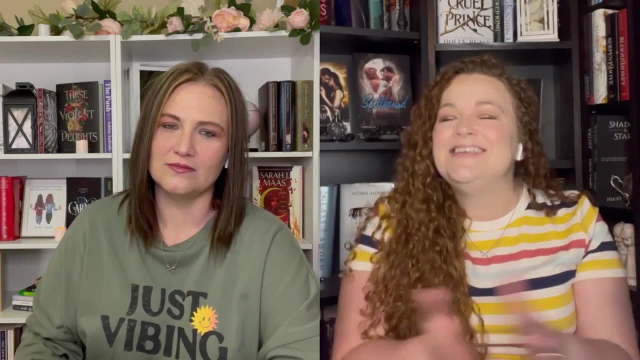 towards poppy were not the best of intentions in the beginning. and of course love came into the picture and it changes everything. but he was doing it for his brother, so hawk is really relatable. i don't know about you guys, but when it comes to my husband, my son, my best friend, my anybody in my 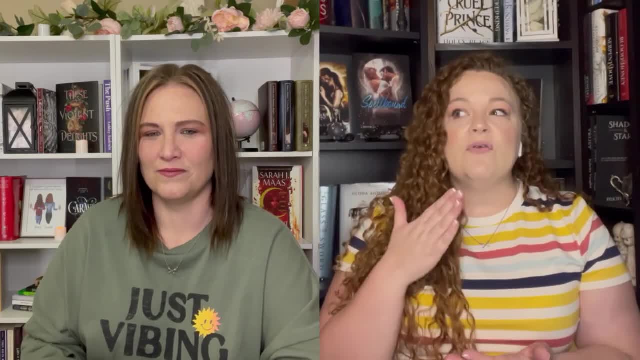 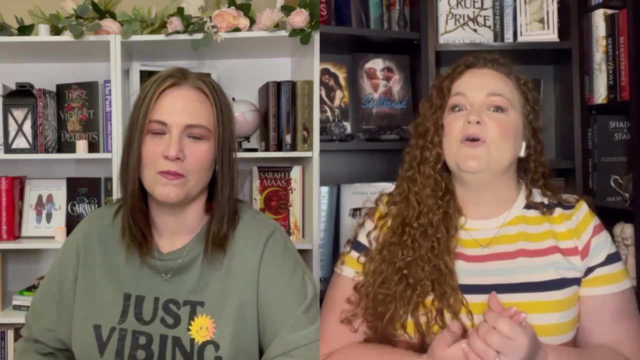 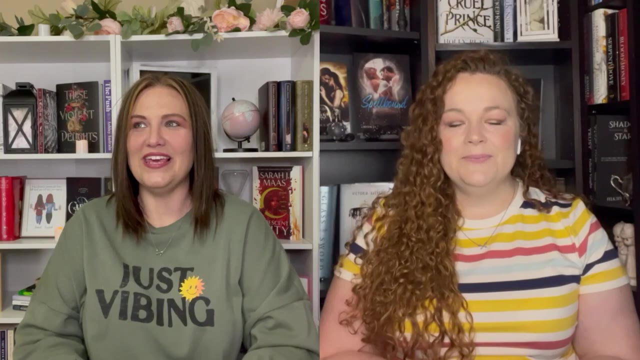 family or my friends. there is a whole bunch of questionable that i would do for them if it meant saving their lives, and that it makes hawk a savageable character living in the gray. the next one: look, i am low-key, high-key, obsessed with aaron warner from shatter me. 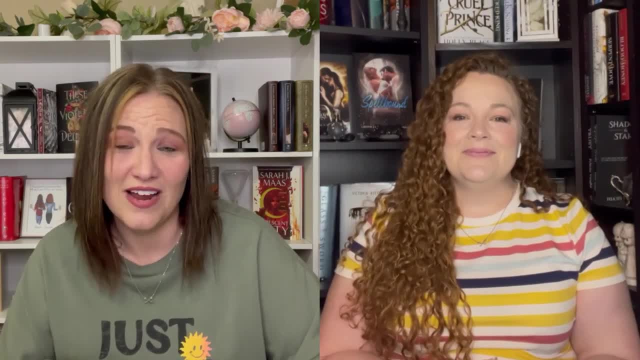 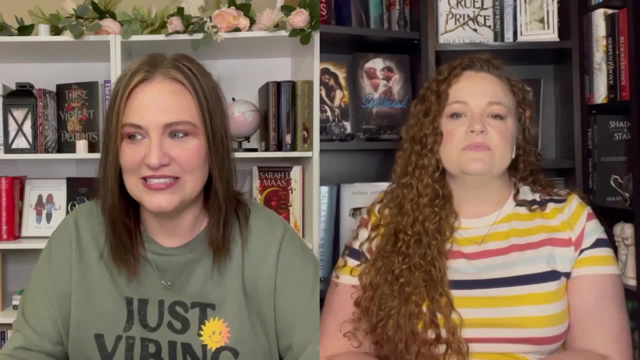 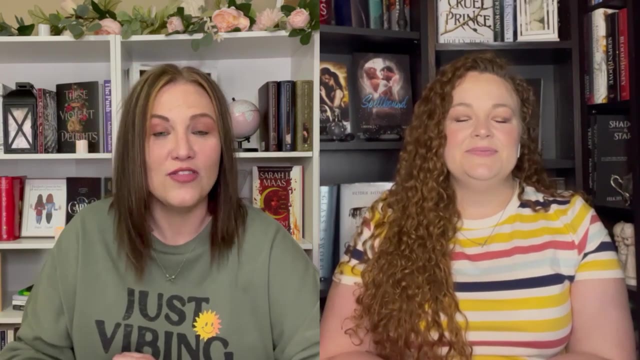 i didn't say adam kent, i said aaron warner. again, if you're still watching and you haven't read it, not sorry. you for the first book and most of the second book absolutely loathe warner. you don't even know his first name. all you know has this warner. you love him. he seems like a psycho killer. 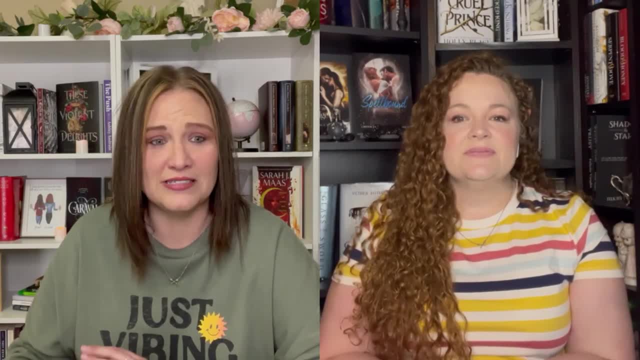 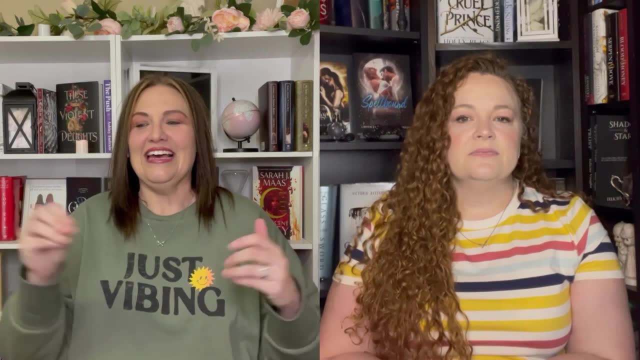 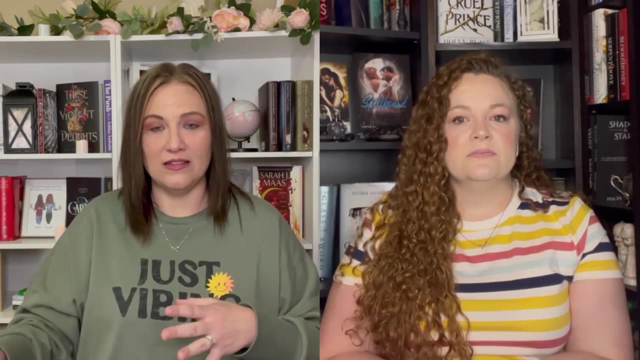 ruthless, just terrible, terrible person. as things start to unravel, there are so many misunderstandings- the king of misunderstandings, for example, he shoots a guy in the forehead and when that happens, juliet, the main character, and the reader- we're all like, oh my god, what? oh my god, you just. 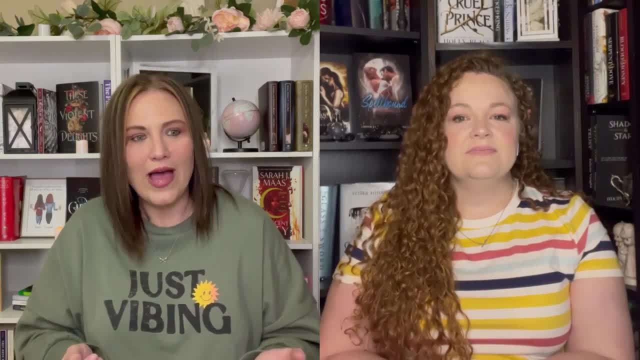 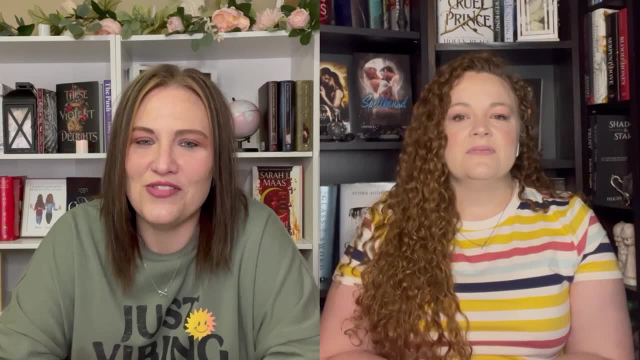 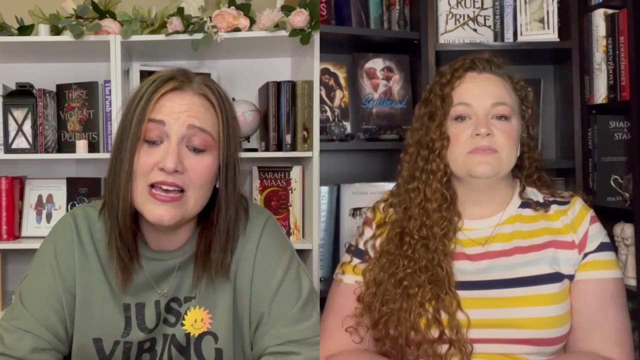 shot that guy in the head for literally like no reason. wow, you're evil. yeah, well, it turns out she calls him out for that later and he puts her right in her place and lets her know that that man was not innocent. he was an alcoholic that was beating his wife and kids on a daily basis. but 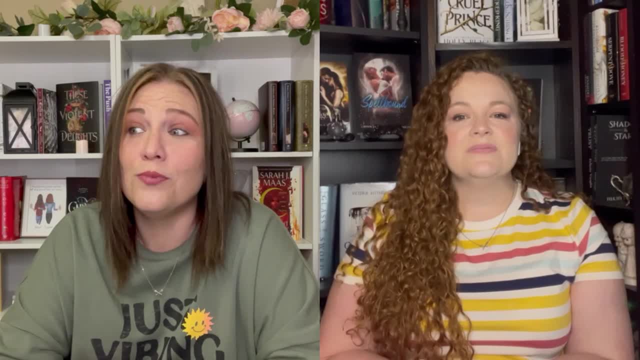 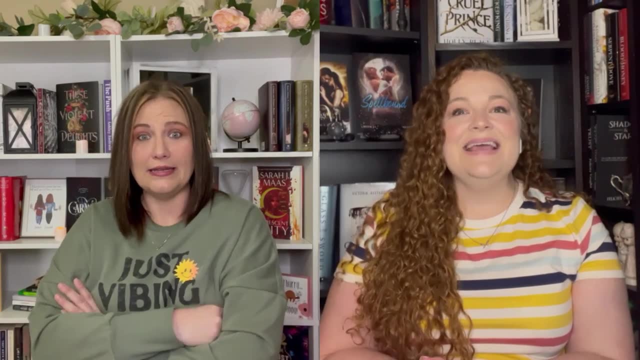 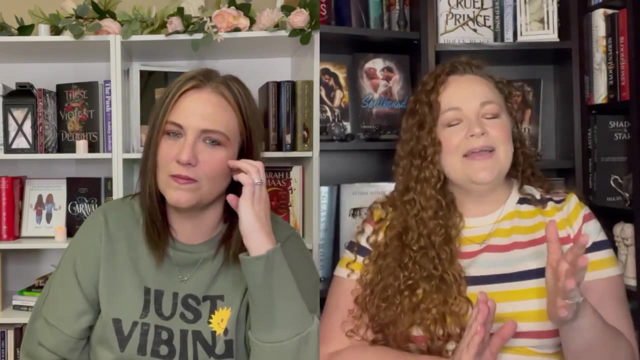 he was so angry that he pushed his wife so hard down the stairs that she lost their unborn child, broke his little girl's arms and legs. like come on okay, yeah, nope, bye. like dude ain't innocent. yes, like so. there are a lot of things that happen like that. the red queen cal, you know you kind of your. 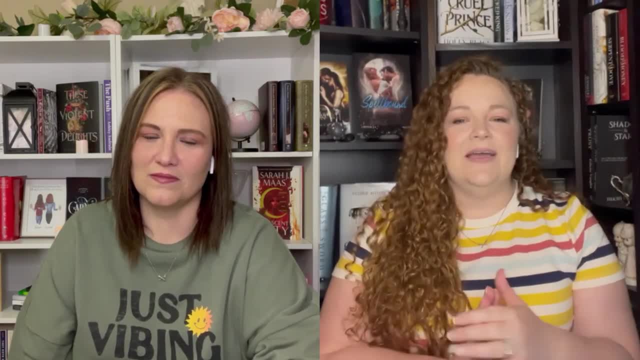 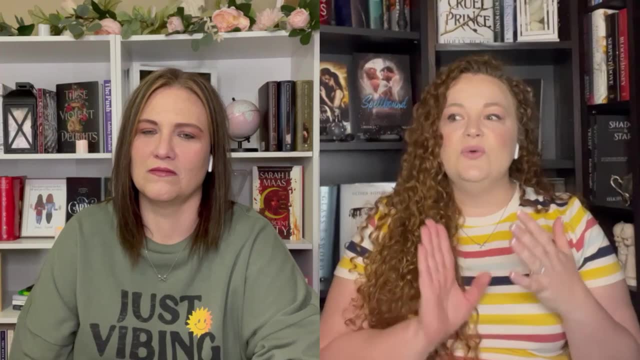 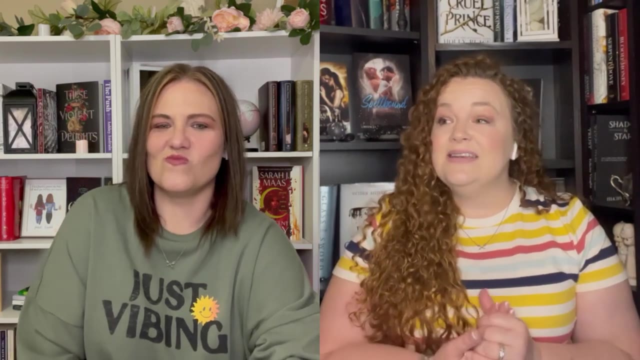 favorite character at the very beginning and you're just like that's the one. cal was that character for me. and cal is set to be king and he is going to run things the way his father did, which is he is an oppressive ruler. he's not the nicest guy. 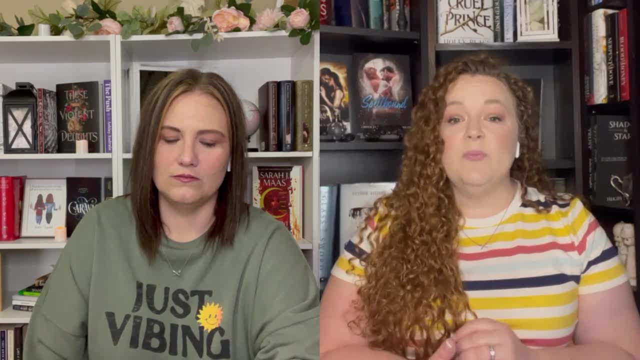 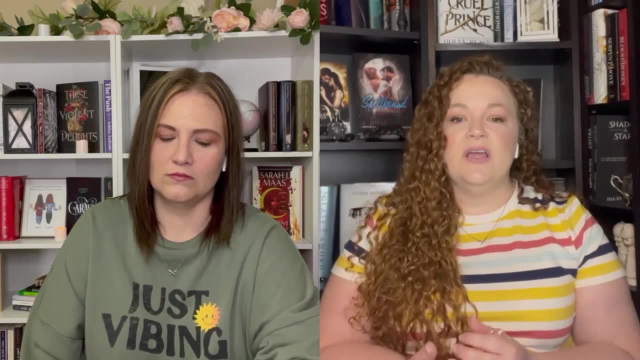 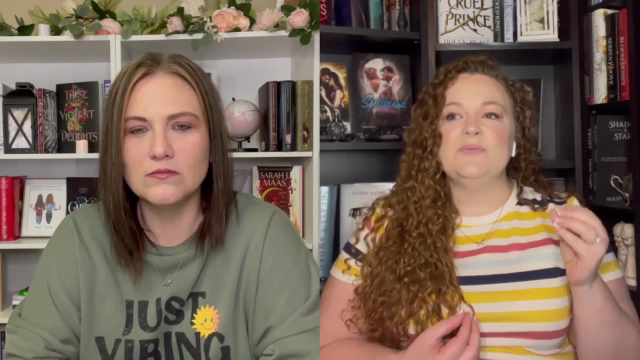 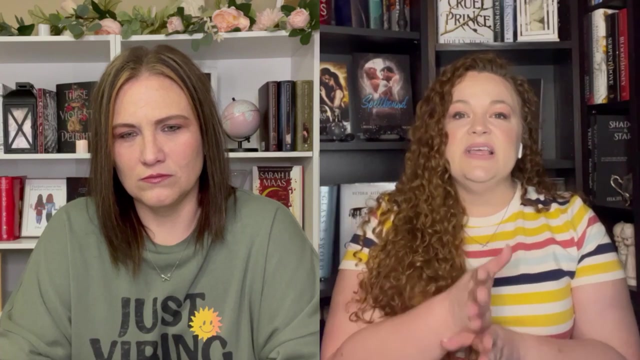 there are people that are looked at as being less of a people because they don't have, you know, powers and and our main character is, at the beginning, one of those people. the thing that makes cal work is between the entire series. cal has an arc and, even as he believes that stuff, as he starts to see mayer change and and do what she's doing. 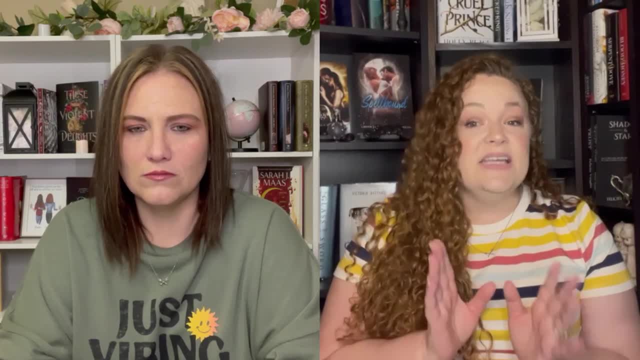 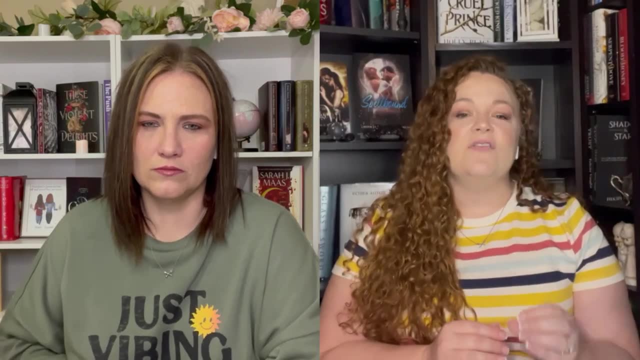 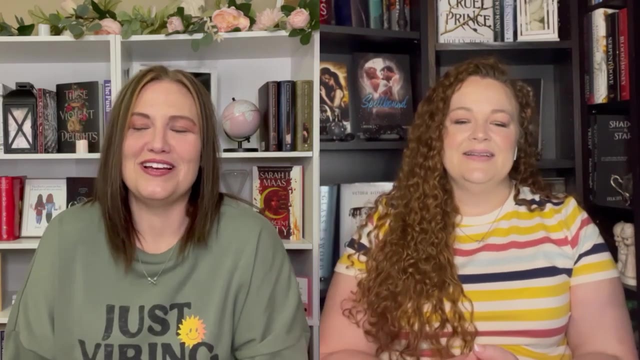 he's moving with her and it's not an easy move for him. he's he's not just like up and up, like cool, let's just go. he fights with this and the character arc for cal really works. this is our only girl on this list. um, and that's lou from serpent and dove. lou, i love lou from the. 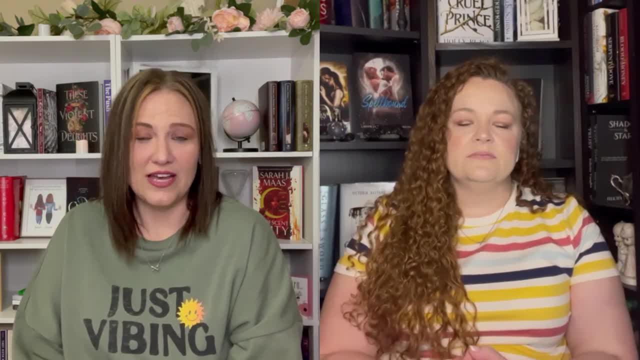 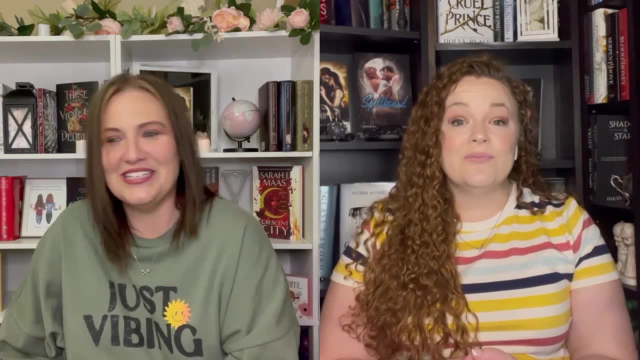 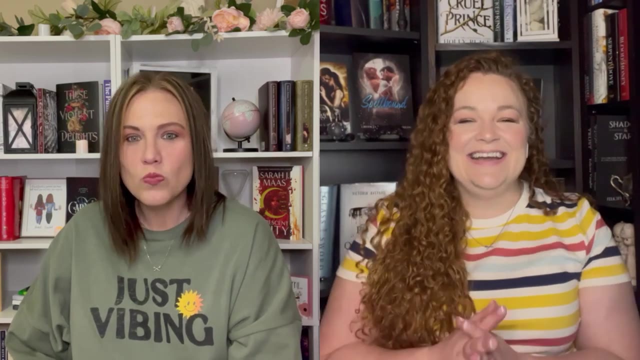 very beginning. i love her character. i never, ever dislike her, but there are times there are things that she does that are morally questionable. i mean, she steals, she kills, she marries a man and doesn't tell him what she is. oh yeah, it's true she lies too, but 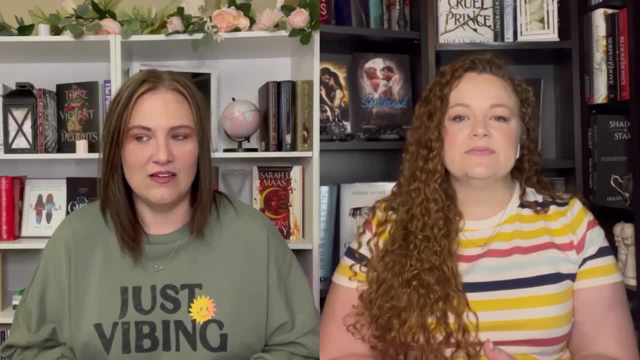 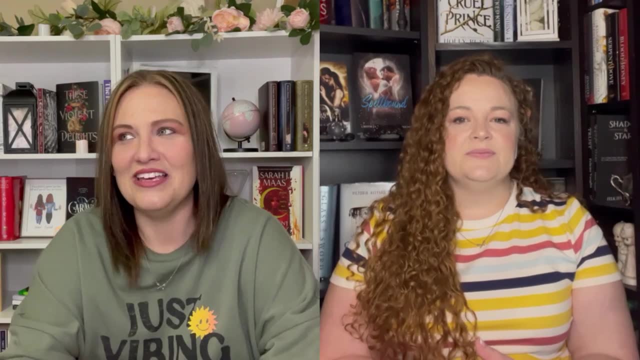 everything she did- the ceiling, the killing- was to protect herself and her, not telling him that she's a witch. that was protecting herself too, because he's a witch hunter. you can look at her as morally gray and questionable, but it love comes along, like you said before, it changes everything last. 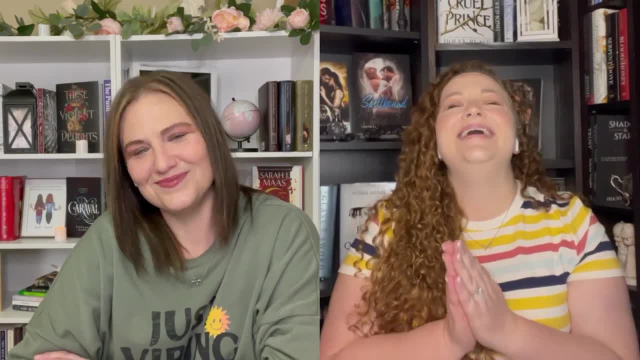 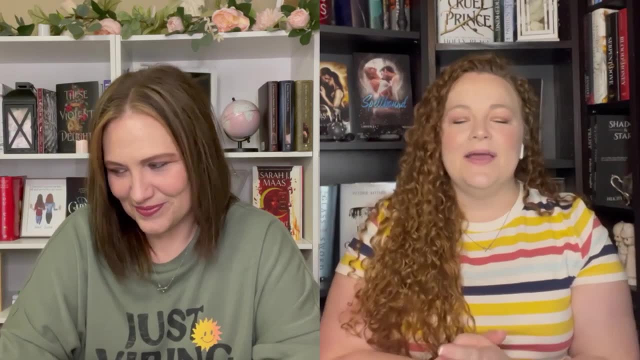 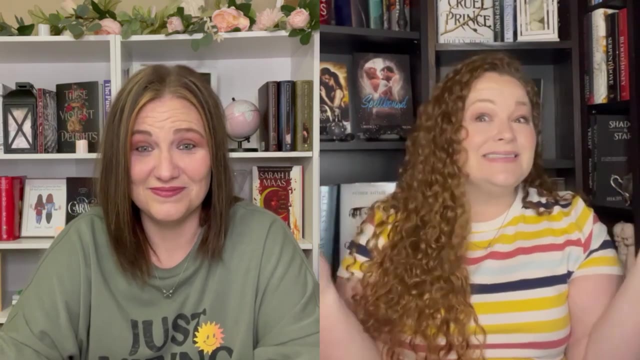 up is carden, our lovely boy with the tell. and no, let's talk about the tail from the cruel prince. i know you either believe the tells air, you just pretend like it's not there. um, so carden is exactly what we're talking about. he's the cruel prince, it? it's right there on the name of the book. 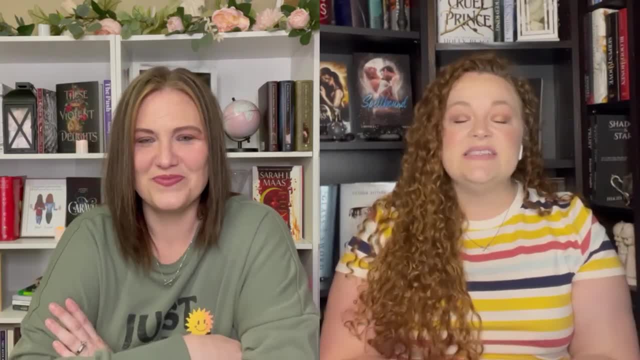 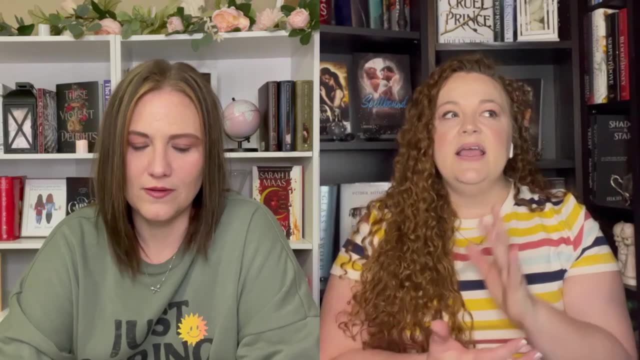 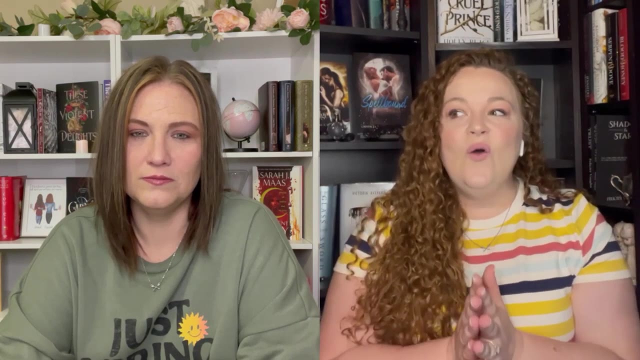 um, he's a dick. he's a dick to jude, he's terrible to jude. and we get into the childhood trauma again. and here's the thing: it's never a it's never a full explanation. you just can't go. well, my main character, my love interest, he went through some childhood trauma and that. 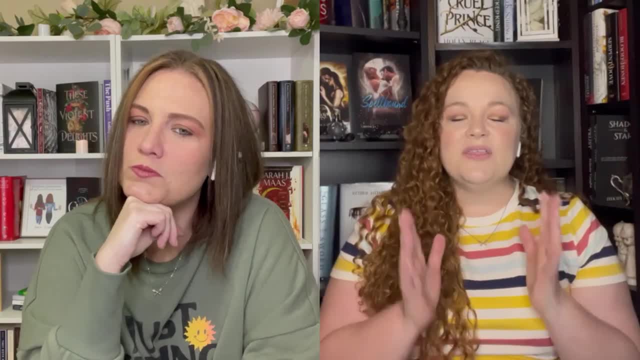 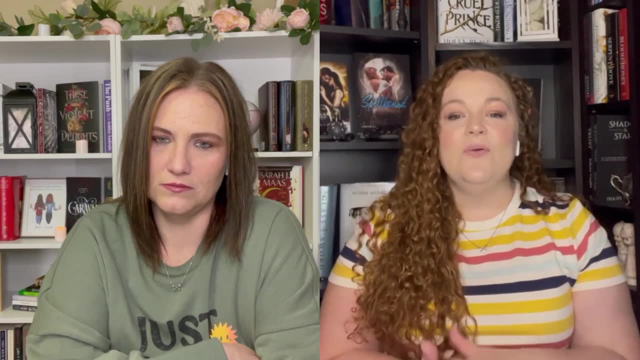 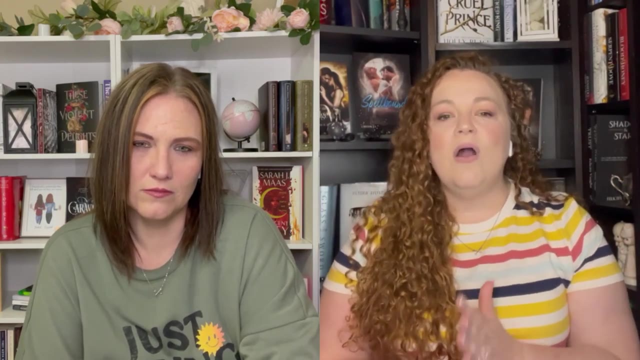 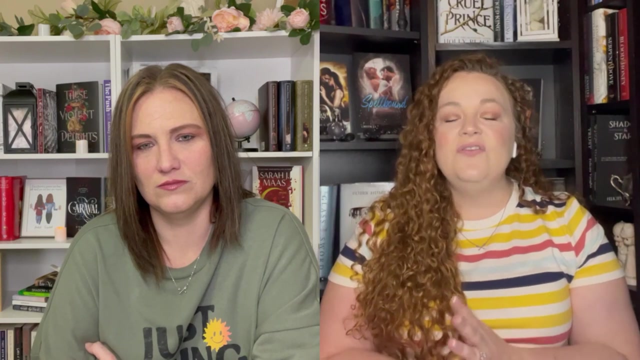 explains everything right. it works with carden, just as it worked with cal, and it works with almost every single one of these other characters is his arc, and who we meet at the beginning with carden and what carden becomes throughout the series changes everything. you fall in love with carden as jude falls in love with carden and you hate carden as jude. 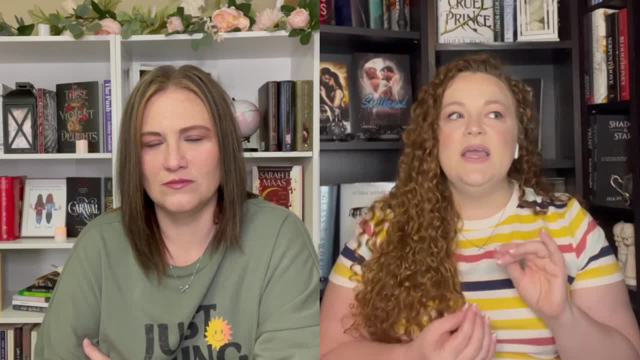 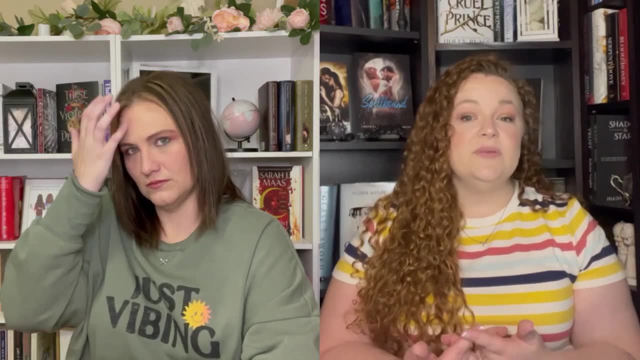 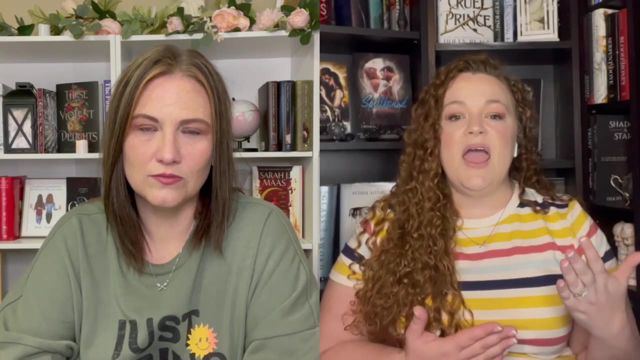 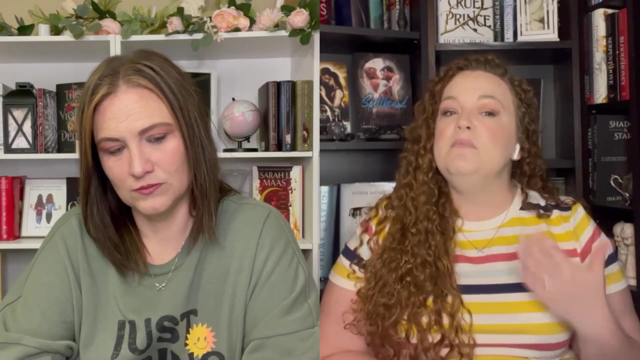 hates carden. so that is really important: to see him pull himself out of the childhood trauma, come and go, and what he's going to be and what he needs to do, and that right there it makes him so human and so relatable that we can let him go for really some really terrible, mean things.